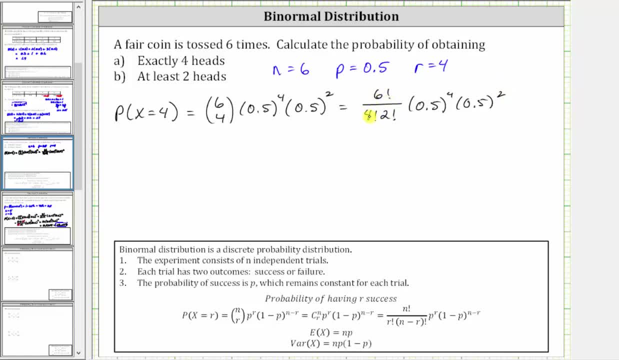 Let's go ahead and simplify this quotient Here, because we have a four factorial in the denominator. let's write six factorial as six times five times four factorial, all over four factorial times two factorial Here, because the bases are the same and we're multiplying. 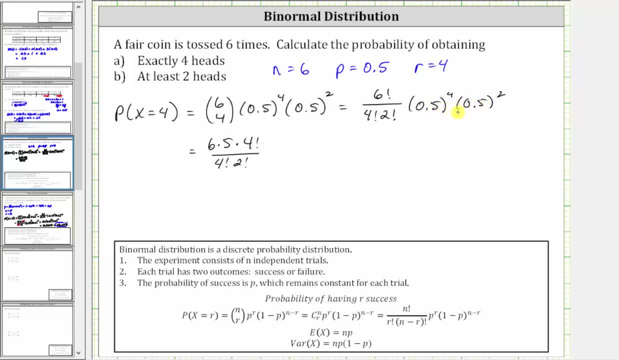 we can add the exponents 0.5 to the fourth times 0.5, squared is equal to 0.5 to the sixth. Simplifying four factorial divided by itself simplifies to one, leaving us with 30.5 squared. 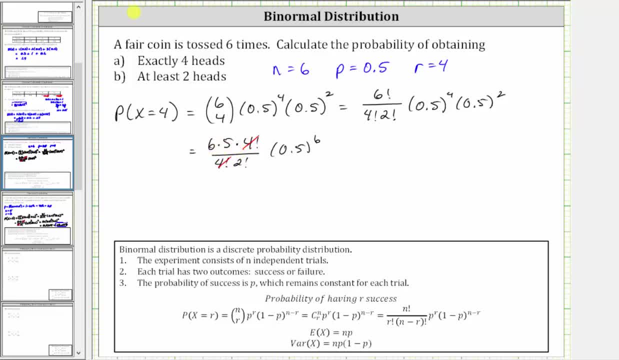 divided by 2, factorial, which is equal to 3 divided by 2 or 15.. This is equal to 15 times 0.5 raised to the sixth. And now we'll go to the calculator: 15 times 0.5. 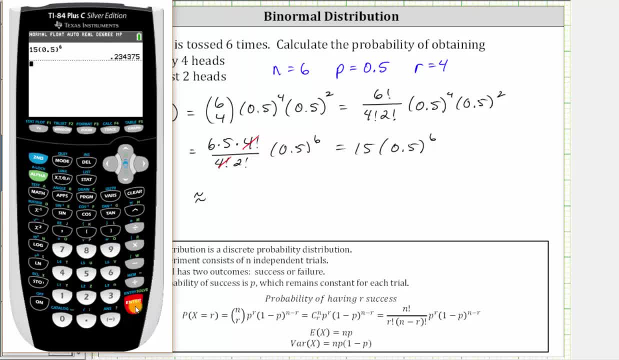 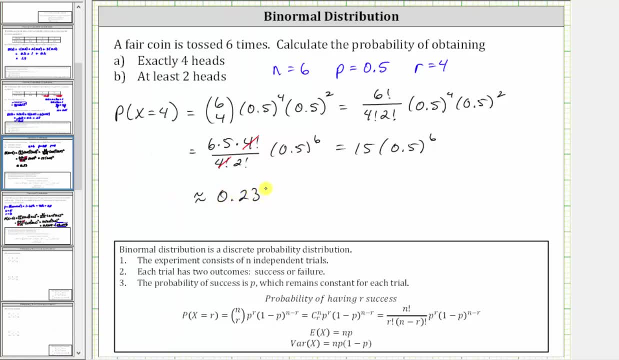 raised to the sixth, rounded to four decimal places, is approximately 0.2344, which is equal to 23.44 percent. So if a fair coin is tossed six times, the probability of getting exactly four heads is approximately 23.44 percent. 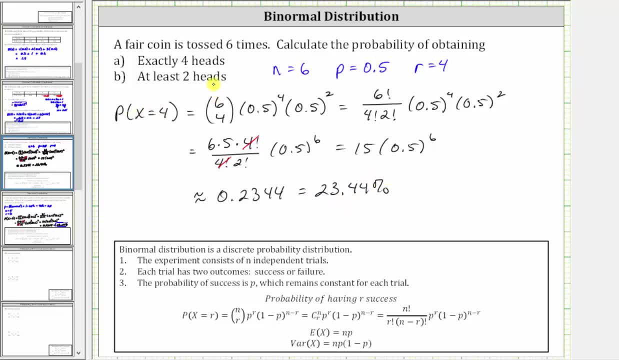 And now let's determine the probability of at least two heads. The probability of at least two heads is equal to the probability x equals 2 plus the probability x equals 3 plus the probability x equals 4 plus the probability x equals 3.. 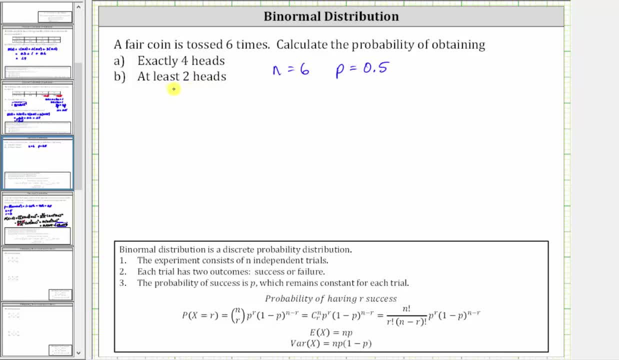 5 and then finally, plus the probability, x equals 6.. It'll be easier to determine the probability of at least two heads by using the complement. So the probability that x is greater than or equal to 2, meaning greater than or equal to two. 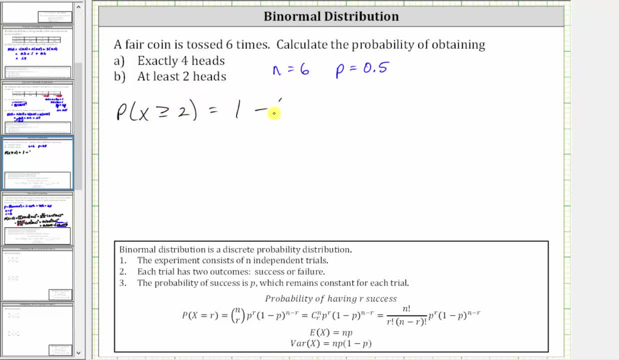 heads is equal to 1 minus the sum of the probability that x equals 0 and the probability that x equals 1.. So again we're saying here: if we take 100 percent and the probability that x equals 1 is greater than or equal to 2, then x equals. 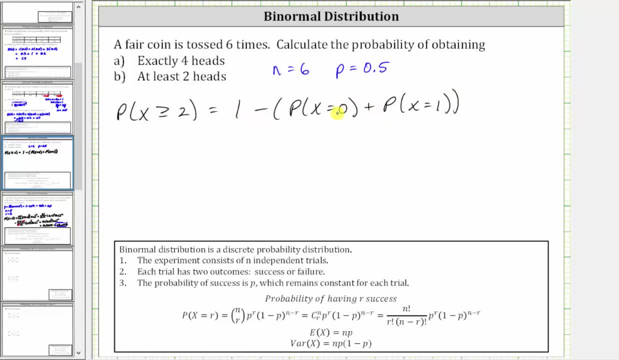 0. And then subtract the sum of the probability x equals 0 and the probability x equals 1, this will leave us with the probability that x is greater than or equal to 2.. And for the probability x equals 0, we know r the 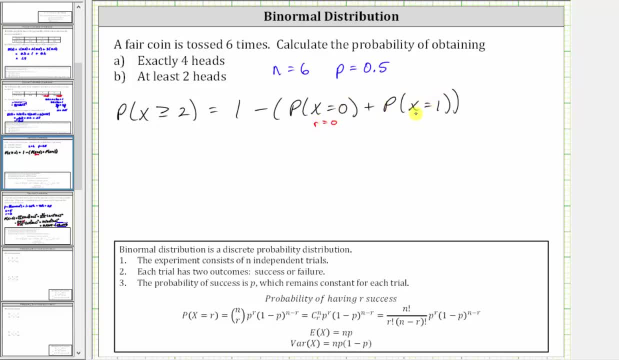 number of successes is equal to 0. And for the probability x equals 1, the number of successes r is equal to 1.. So this is equal to 1 minus again the sum of these two probabilities. With the probability x equals 1, the number of successes r is equal to 1.. So this is equal to 1 minus again the sum of these two. 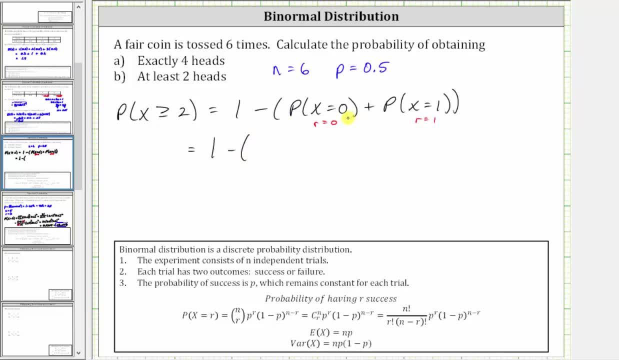 probabilities where the probability x equals 0 is equal to 6, choose 0 times p raised to the power of r, which is 0.5, raised to the power of 0, times the quantity 1 minus p raised to the power of n minus r, which is 0.5 to the sixth, and then we: 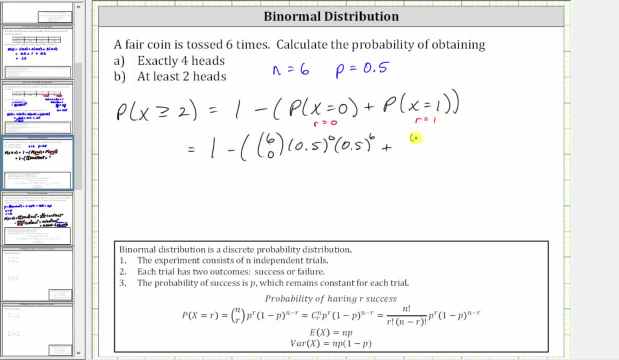 have, plus the probability, x equals 1, which is 6. choose 1 times 0.5, raised to the power of 1 times 0.5 raised to the power of n minus r, which is 5. and now let's find these two probabilities. we have 1 minus 6. choose: 0 is 6 factorial. 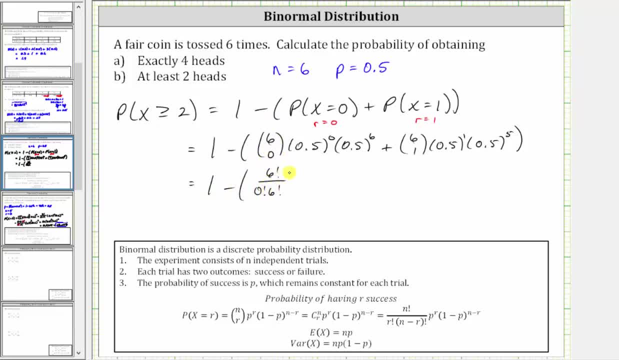 divided by the product of 0 factorial and 6 factorial, and 0 points five to the zero is equal to one, so we have 0.5 to the sixth plus 6, choose 1 is equal to 6 factorial. divided by the product of 1 factorial and 5 factorial. 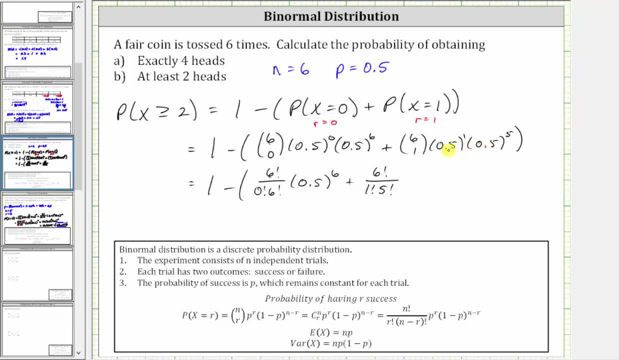 and here, because we're multiplying, the bases are the same. we can add the exponents. this product is 0.5 to the sixth, let's continue simplifying. we have 1 minus 6 factorial divided by itself. simplified simplifies to one. zero factorial is equal to one. 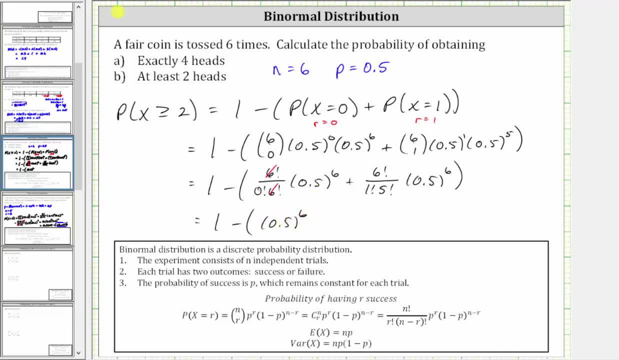 and therefore we just have 0.5 to the sixth, Because we have a five factorial here. let's write six factorial as six times five factorial, and then we have divided by one factorial times five factorial. Well, five factorial divided by itself simplifies to one. 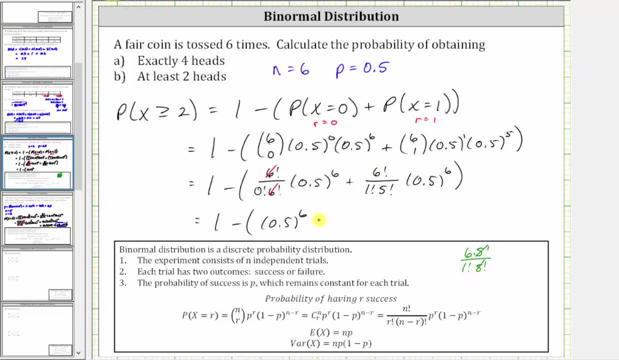 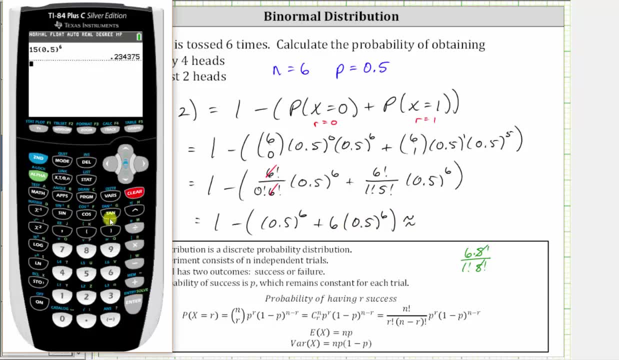 One factorial is one and therefore this simplifies to six and then times 0.5 to the sixth. And now let's go to the calculator. We have one minus and then in parentheses, we have 0.5 raised to the power of six.